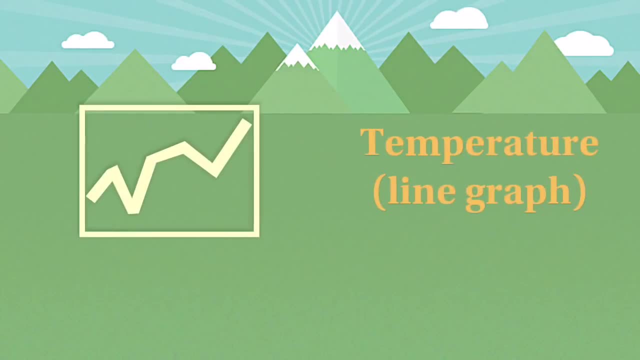 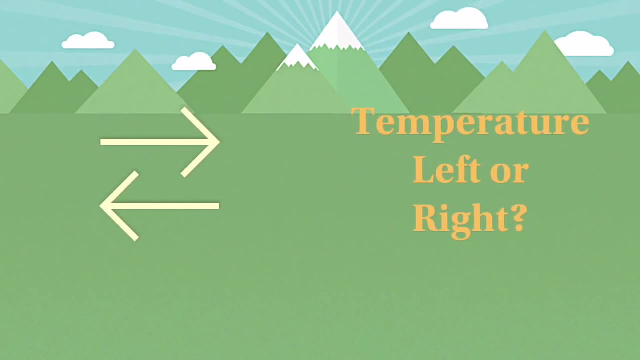 looks like rainfall. so that's the graph to use. Then, for temperature, just use the other graph. Now I've done some research and I've been unable to find a definitive answer as to whether the temperature or rainfall should be on the left or the right of the graph, So I'm going to take 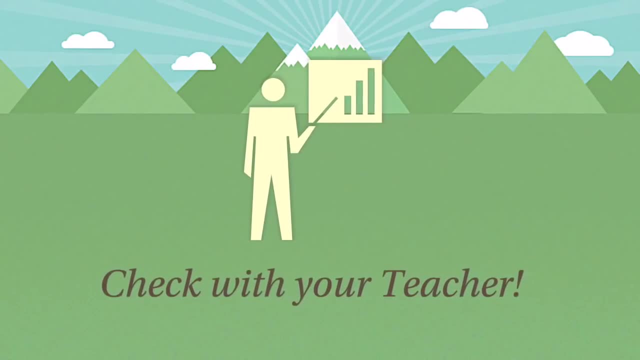 the easy way out and say: check with your teacher which one they prefer For my graph. I'll go: rainfall or precipitation on the left and temperature on the right. Now this is not going to be a perfect looking graph. I've deliberately done it by hand to show you the whole process. 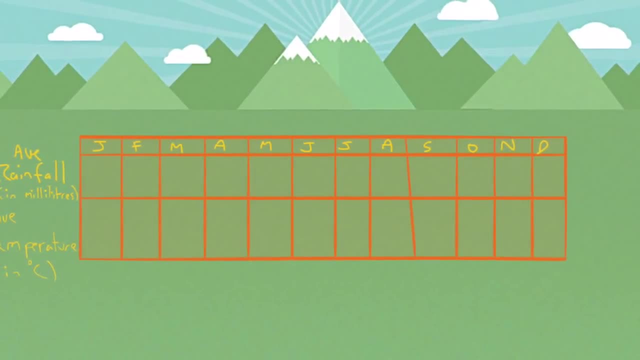 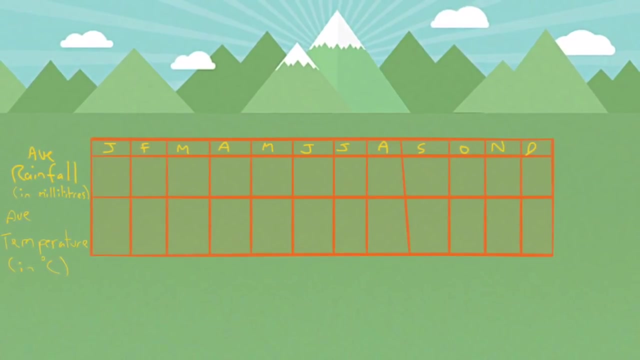 To start you need the data. Usually it'll look something like this, with a table set out with all the months and then average rainfall and average temperature on the side. I've just thrown in some numbers there. They don't actually correlate to the graph. It's just an example of 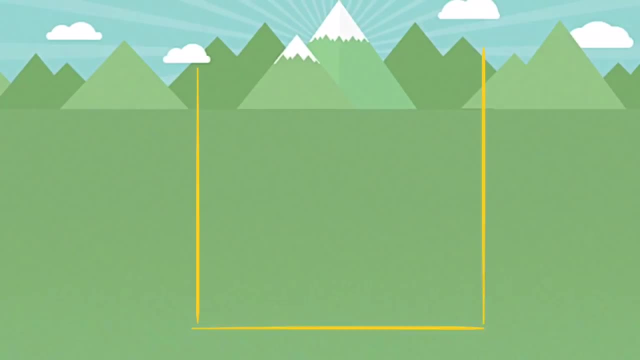 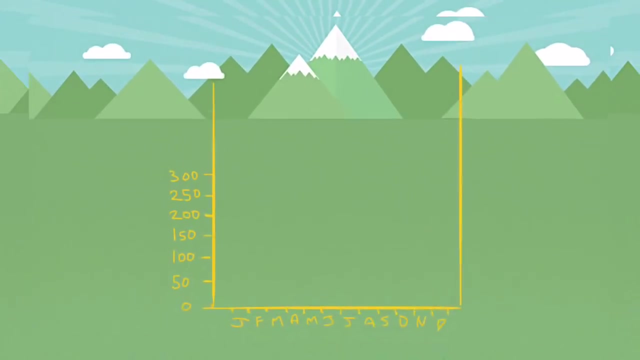 what you'll see: a big square U or, if you prefer, the top half of rugby league or rugby goal posts. Then split this up evenly with the 12 months at the bottom, Then with a ruler, set out even spaces for your rainfall and throw up the numbers on. 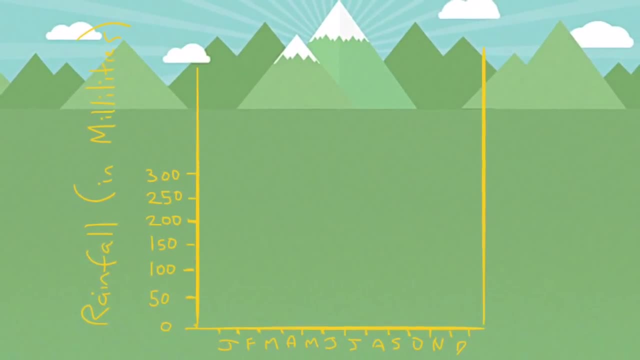 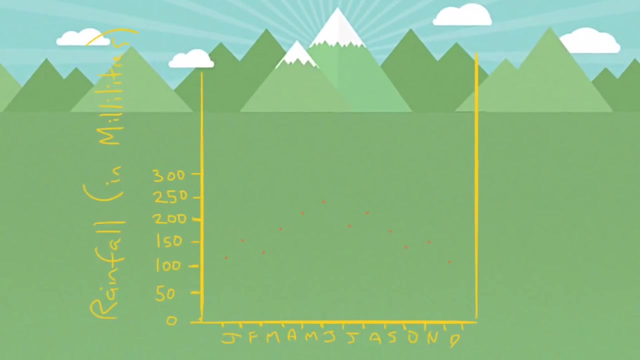 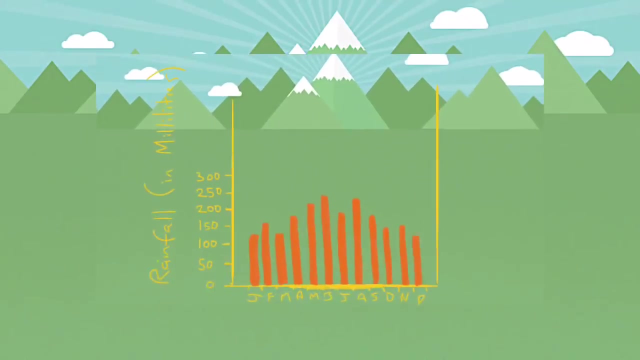 the left hand side. Remember to always include rainfall in millilitres, so that the person reading the graph knows what each number signifies. Once you've done that, grab your ruler and put a dot in the middle of each month exactly where the average rainfall fell for that month. 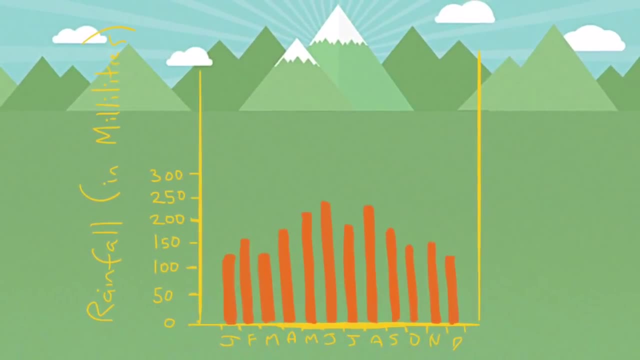 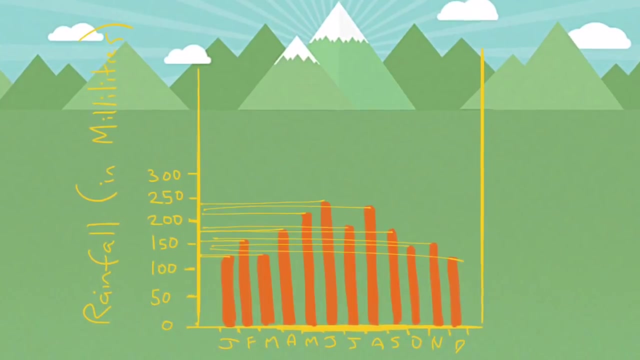 Then complete your bar graph. As I said, guys, I'm not spending a whole bunch of time making this look pretty. Once you've completed this, it's always helpful to double check that you've got your measurements right with the average rainfall for that month. 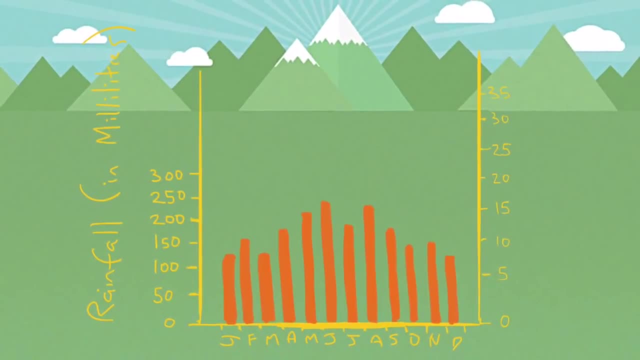 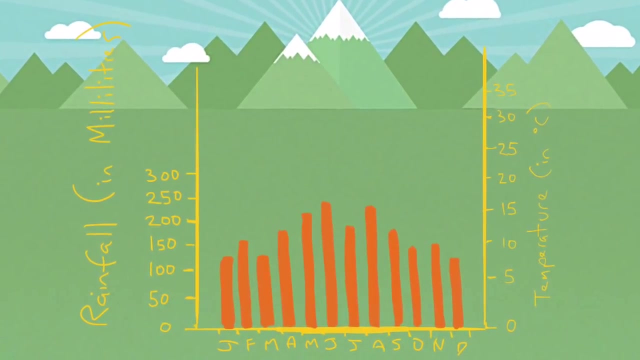 Once you've done this, on the other side of your graph, set out in equal parts the temperature going up the right hand side. Don't forget to write out your measurements. Write out temperature in Celsius so that people know what those numbers signify. 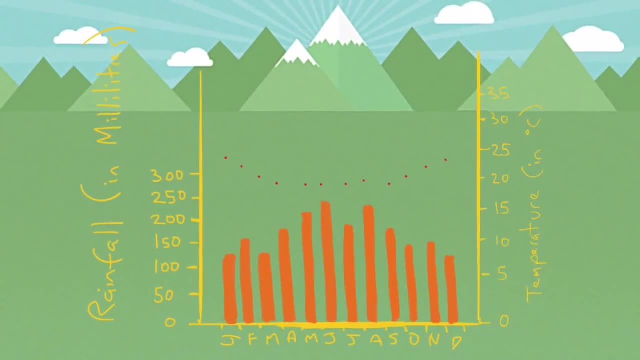 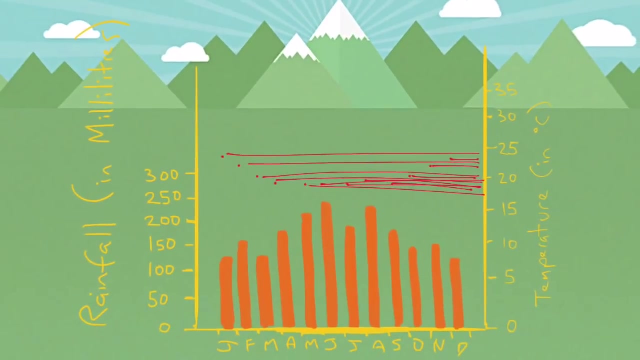 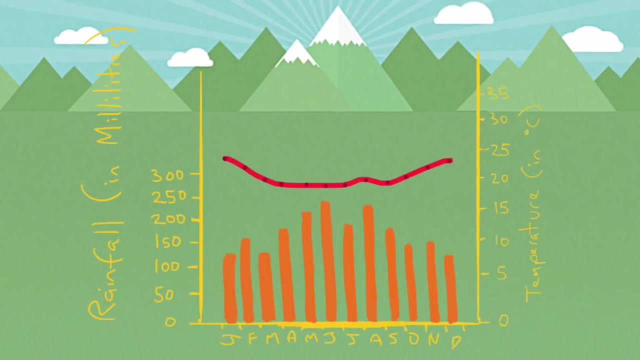 Then, once again with your ruler, plot out for the middle of each month where the average temperature fell. Make sure the dot is right in the middle of each month and exactly equal to where it should be temperature wise. Then plot it out as a line graph with the dots still being visible.